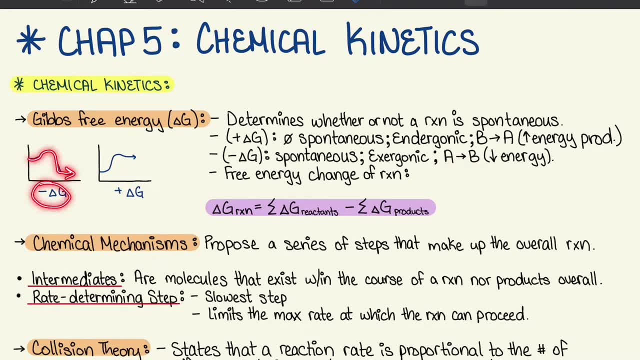 And ends with low energy products. So the free energy change of reaction can be shown with delta G reaction is equal to the sum of the delta G of reactants minus the sum of delta G of products. and that's our equation. Moving on to chemical mechanisms, it proposes a series of steps. 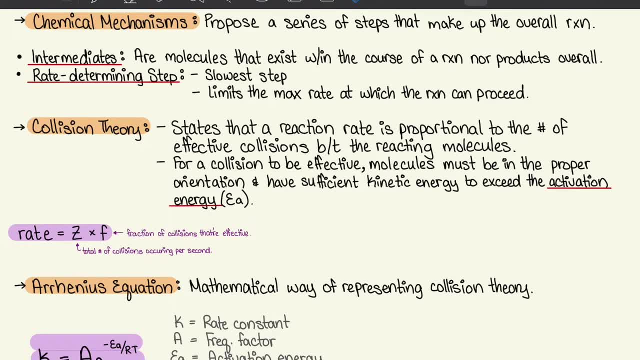 that make up the overall reaction. So the intermediates that we have are molecules that are within the course of a reaction, nor products overall. And the rate determining step is the slowest step and limits the max rate at which the reaction can proceed. So intermediates are the ones. 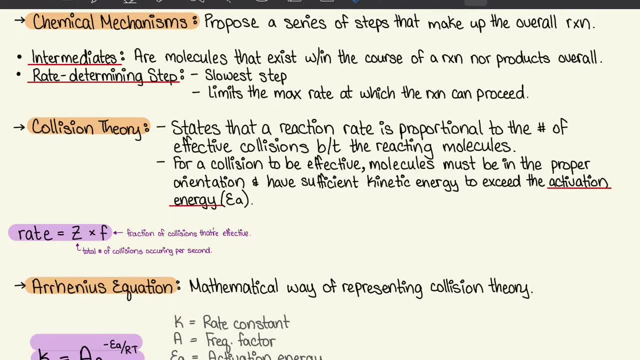 that if, when we were to add products get cancelled out, so they're just intermediate, they're not in the final overall reaction. Moving on to collision theory, it states that a reaction rate is proportional to the number of effective collisions between the 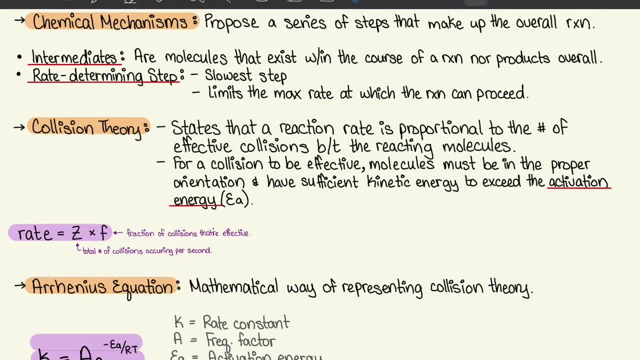 reacting molecules. For a collision to be effective, molecules must be in the proper orientation. number one and number two must have sufficient kinetic energy to exceed the activation energy which is written with EA And the equation we have for that is: 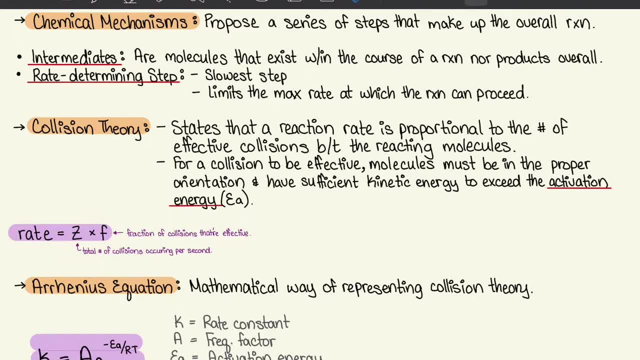 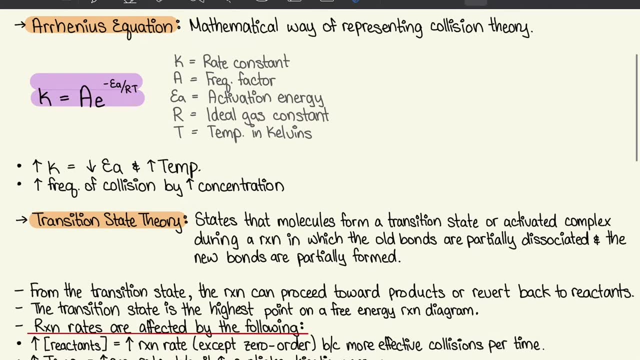 rate is equal to Z times F, where Z is the total number of collisions occurring per second and F is a fraction of collisions that are effective. So this is an important equation to keep in mind And when we move forward to the Arrhenius equation, it's a mathematical way to represent. 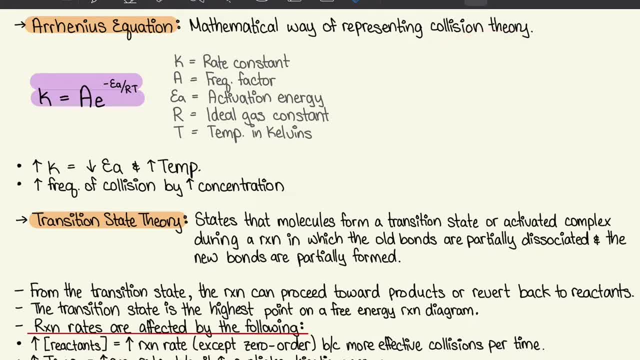 the collision theory that we just talked about. So we have: K is equal to AE, to the power of negative EA, which from before we know is activation energy over RT. So K is equal to the rate constant. A is the frequency factor, EA is the activation energy, R is the ideal gas. 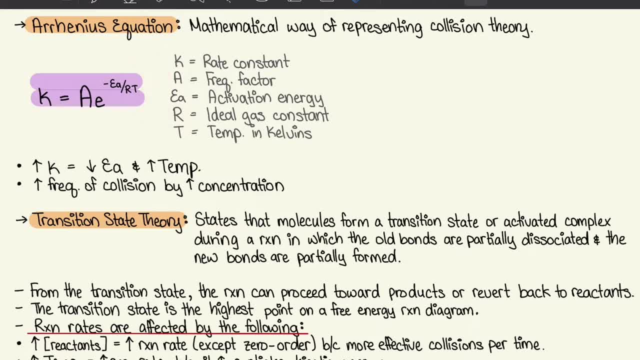 constant and T is the rate constant. So we have: K is equal to the rate constant. A is the temperature in kelvins. One thing to keep in mind is as you increase K, you will decrease EA and increase the temperature. So make sure you know the relationship between the different. 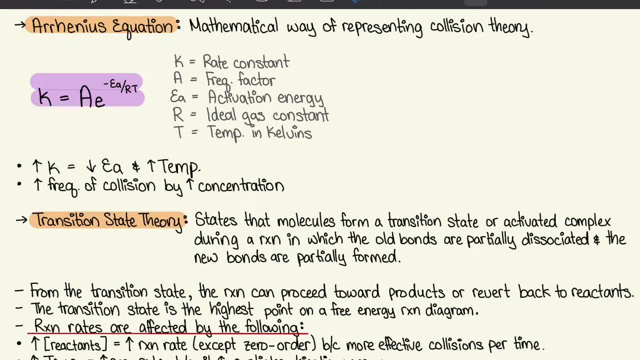 components in this molecule And you can increase the frequency of collisions by increasing the concentration, which makes sense. So the more molecules of a certain element there are, the higher the chances of them colliding. After this, we'll move on to the transition. 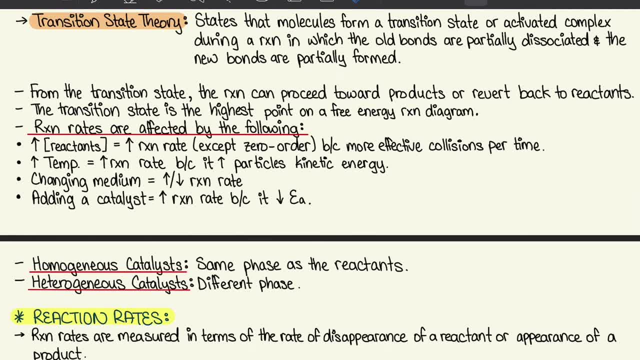 theory which states that molecules form a transition state or an activated complex during a reaction in which the old bonds are partially dissociated and the new bonds are partially formed. So this is kind of the middle state, where it's not fully formed but it's not. 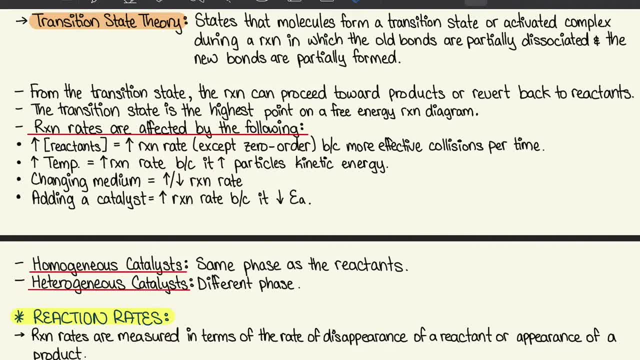 fully dissociated as well. So from the transition state the reaction can proceed towards products or revert back to the reactants. The transition state is the highest point on a free energy reaction diagram And the reaction rates are affected by the following. So if you increase reactants, you'll 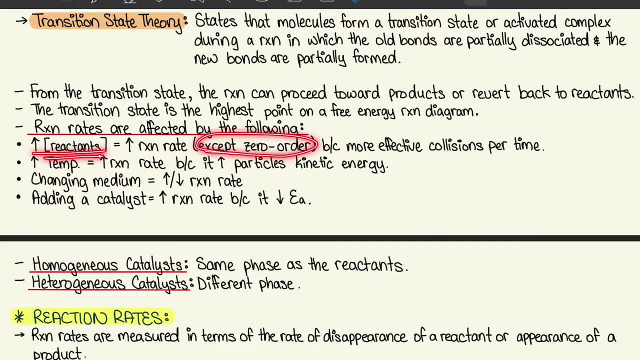 increase the reaction rate except zero order, because more effective collisions per time. And if you increase the temperature you also increase the reaction rate because of high particles, kinetic energy, And another one is changing the medium. So depending on what medium they're in, if they're easy to flow in this particular medium you're going to. 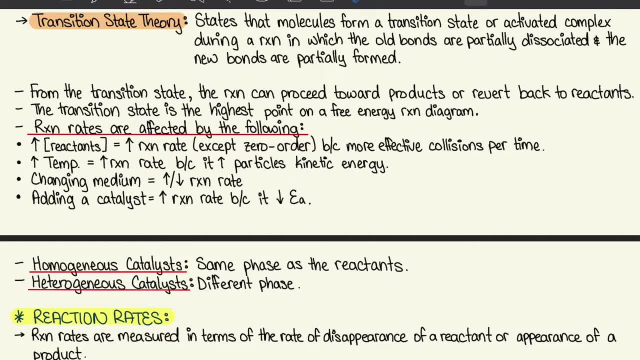 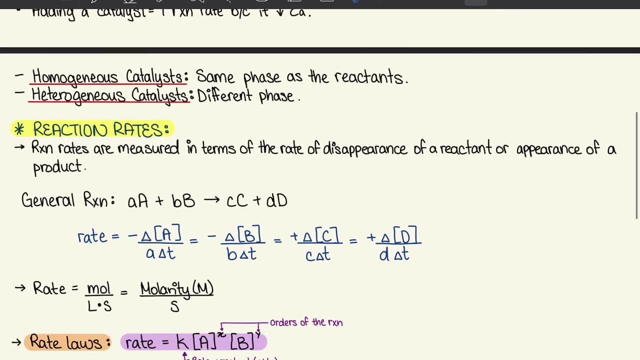 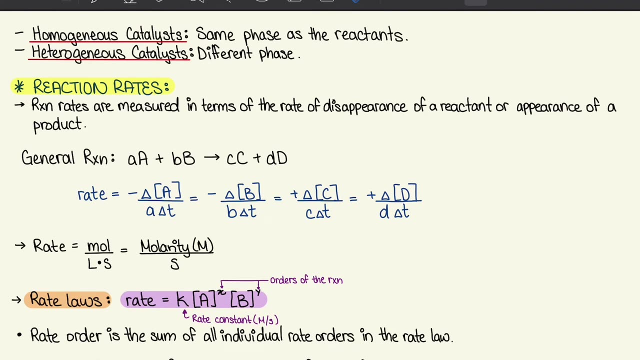 add more materials, theming in a medium that will make the reaction a little more impossible for Mexican catalysts, you're going to cancelling the movement. Next, we're going to move on to 5.2, where we talk about the reaction rates. 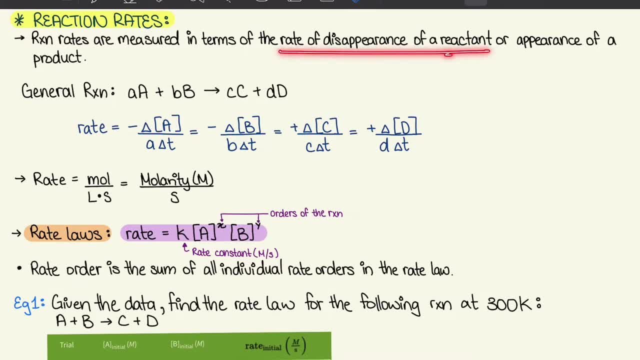 Reaction rates are measured in terms of the rate of disappearance of a reactant or an appearance of a product. In this general reaction equation, the lowercase letters are the coefficients and the uppercase letters are the concentration of the different molecules that may be present. This is an equation we can use to determine the rate for the different concentrations. 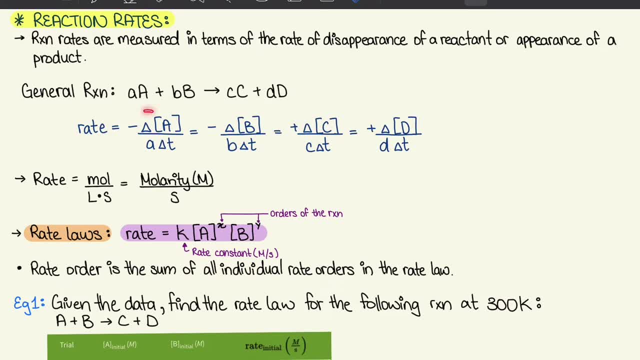 Just take note that the reactants have a negative sign in front of them, whereas the products have a positive sign and they're over the coefficient times. the time Rate is equal to moles over liters per second, and moles per liters is actually molarity. 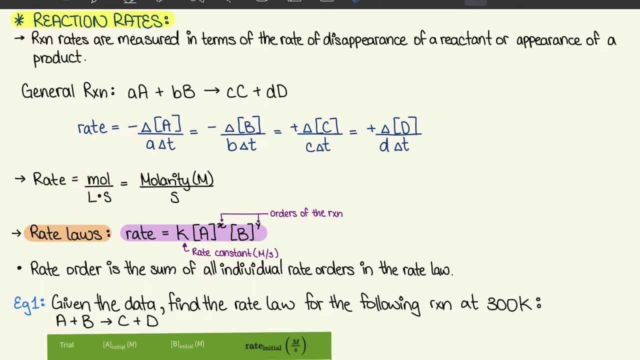 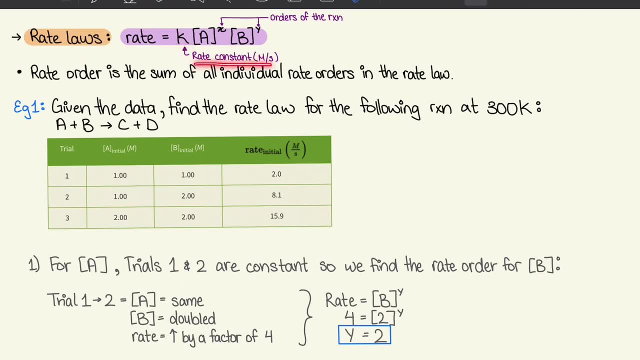 so it's capital M over s for seconds. So, moving on to the rate laws, we have an equation where rate is equal to k, which is the rate constant, and that's molarity over second, like we talked about before, with the concentration of the products and the x and y being the orders of this reaction. 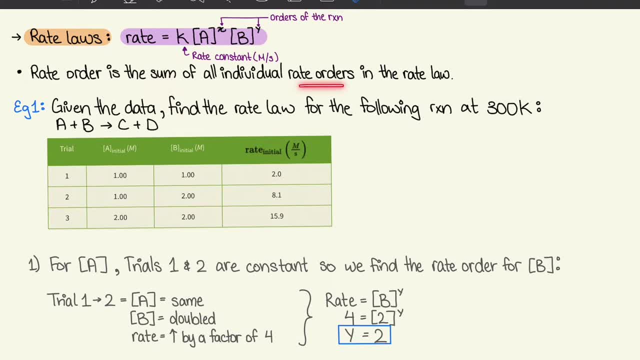 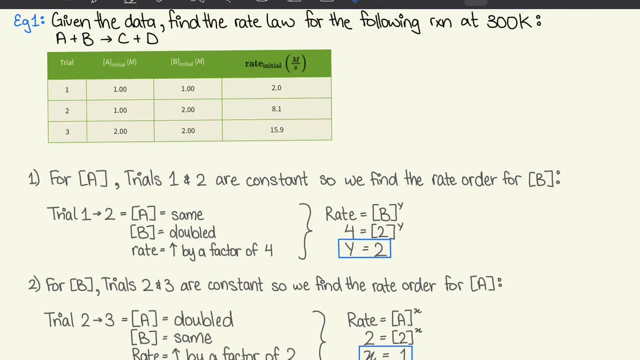 So the rate order is the sum of all individual rate orders in the rate law reaction. Here is an example. So, given the data below, find the rate law for the following reaction: S300.. 300 Kelvin. So A plus B is equal to C and D. so we know that A and B are reactants. 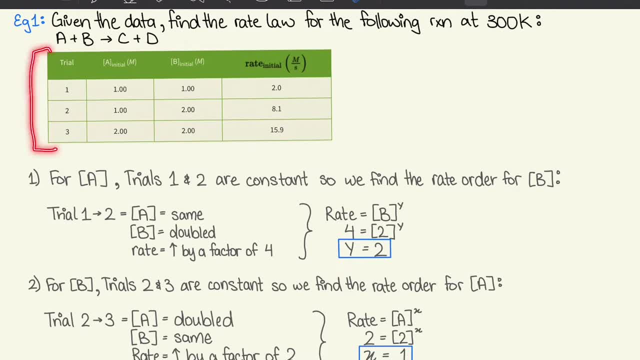 And in this table we're given the initial concentration values for A, B and we're given the rate initial value as well. So what we're told is to find the rate order. So the first step is for the A concentration. we're going to use trials 1 and 2 because they 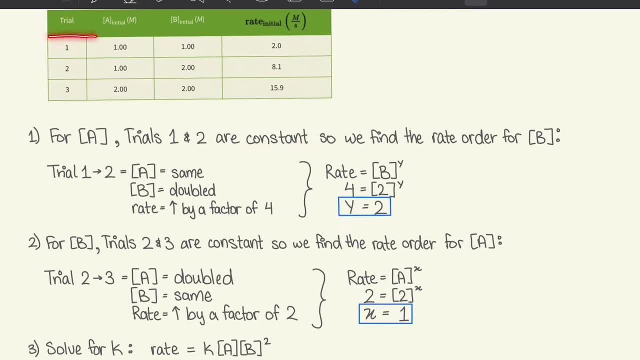 are constant, So we can find the rate order for B. Because they're constant, we don't need to worry about it, and we look at the difference on how that affects the concentration for B. so that's why we do it this way. So for trial 1 to 2, we know that the concentration of A is the 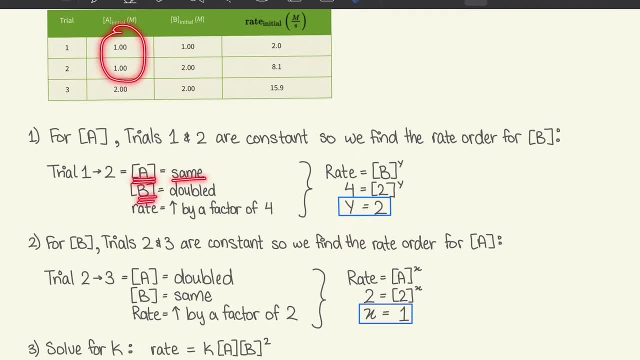 same, but the concentration of B doubles, where it goes from 1 to 2.. And when we look at the rate, we see that it goes from 2 to 8 approximately, So that increases by a factor of 4.. And we're just going to write: rate is equal to B to y. 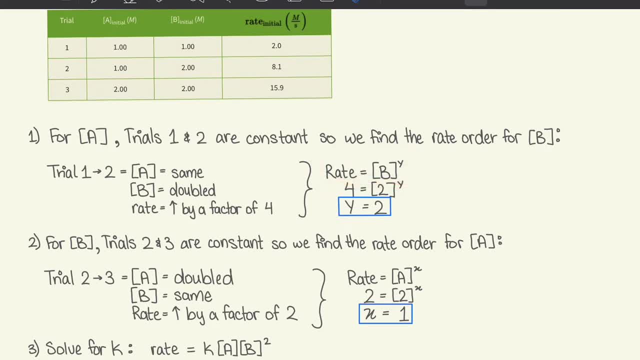 where y is the rate order. So we know that rate increases by a factor of 4, so we're going to write 4.. And we know that the concentration of B doubles for this, so we're going to write a 2 there. And when we solve for y, we get y is equal to 2.. So the rate order for B is 2.. 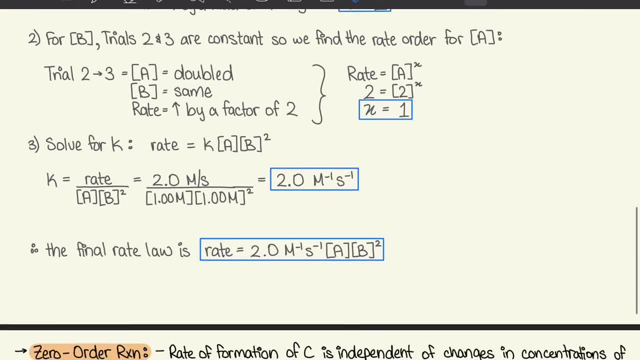 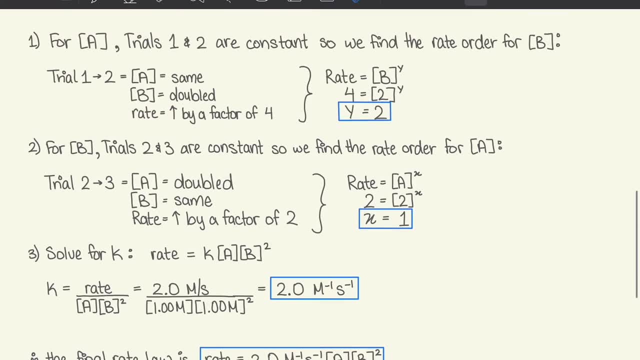 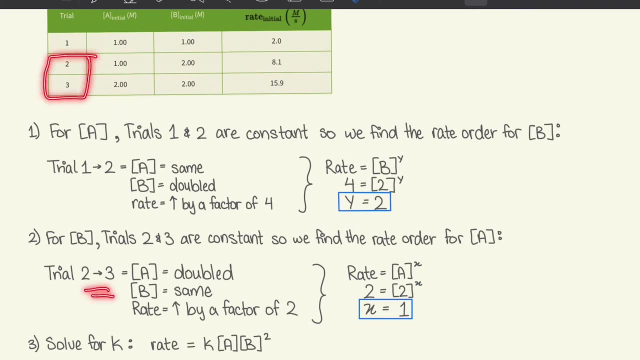 Now to find the rate order for A, we're going to use the two constants for Bs, Because B stays the same and that's our neutral or null value. we're going to use trials 2 and 3 to find the rate order for A. So for trial 2 and 3, we know that A doubles where it goes from 1. 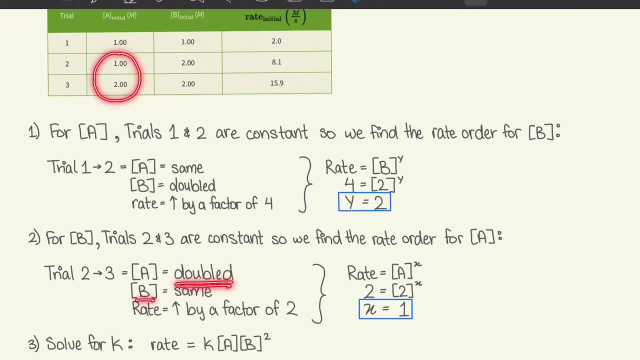 to 2.. And we know that the concentration of B stays the same because it's 2 and 2.. When we look at the rate concentrations, it goes from 8 to approximately 16.. So we can say that it increases by a factor of 2.. And once again, we're going to write out this equation on the side here. 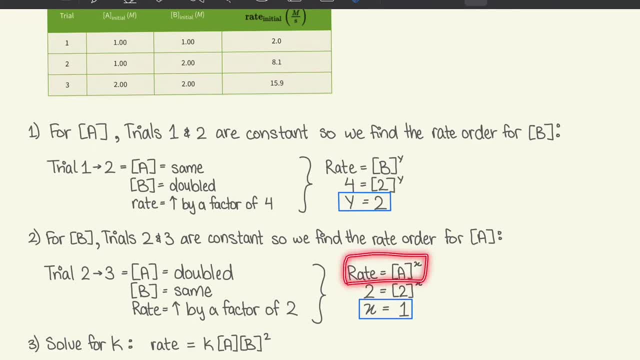 where rate is equal to A, to the value of x, and x is the rate order for the concentration A. So we know that rate increases by a factor of 2, so we're just going to write 2 there. And A is doubled, so we're going to write 2 there as well. 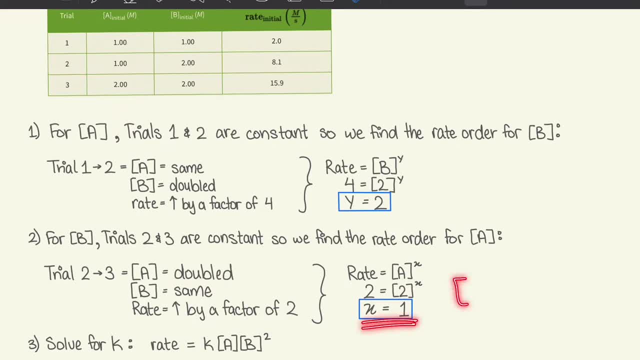 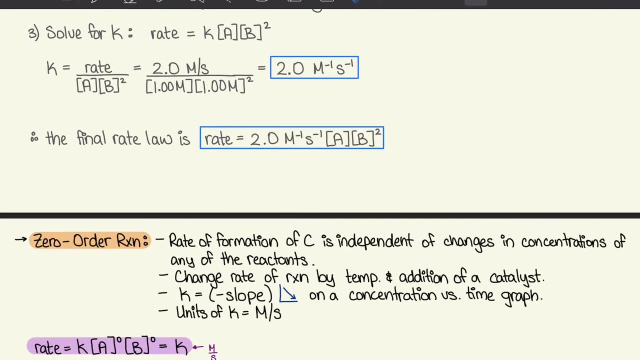 For x, it's going to be 1.. So the third step is to solve for k, And we're going to use the rate equation, like we said before, Because we know that the rate order for A is 1, and the rate order for B is 2,. 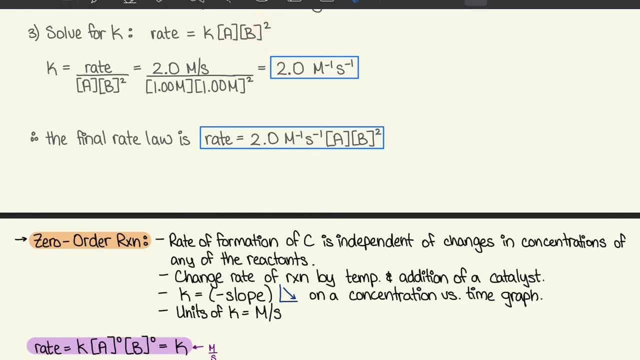 we're going to write those in, We're going to rearrange the equation and solve for k. We're going to input the values from any single trial that we like, And for this I chose trial number 1.. Just simple. So we have concentration of A, which is 1, concentration of B, which is 1 squared. 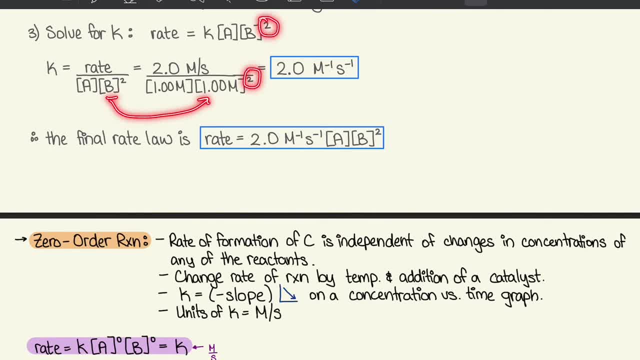 because we know that the rate order for the B concentration is 2.. And then for rate, we're going to go with 2.. Once we solve all of that, we get 2.01 over molarity times second. So therefore the final rate law is: rate is equal to 2.0, m to the negative 1,, s to the negative 1,. 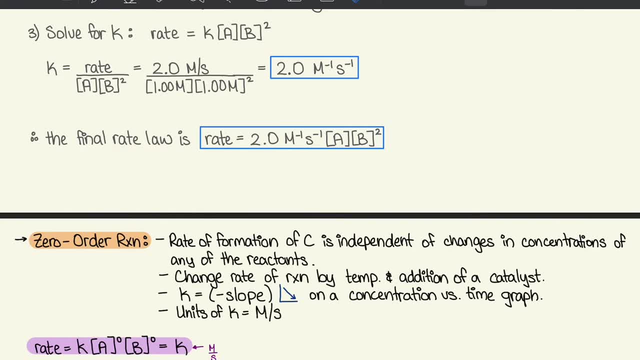 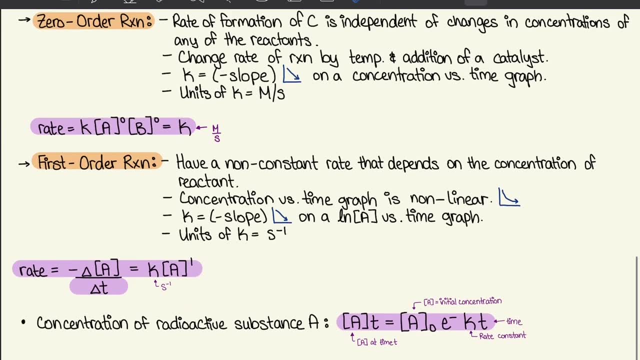 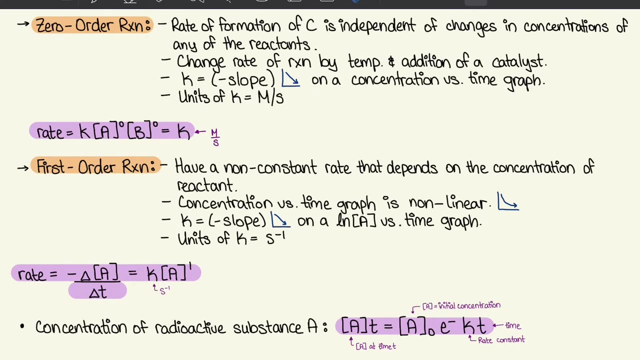 A concentration with the order of 1, and B concentration with the order of 2.. And that's our final answer. So zero-order reaction is the rate. formation of C is independent of changes in concentration of any of the reactants. So for the zero-order reaction the change rate of reaction is by temperature or addition of a catalyst. 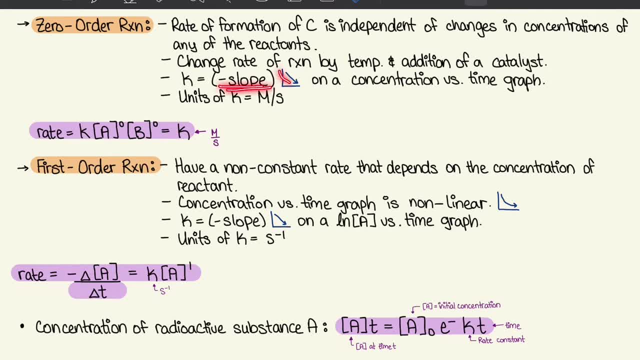 And the k value is a negative slope on a concentration versus time graph where the units of k are molarity plus per second, And that's the equation below. So when we put the zero-order for each, anything to zero is equal to one. 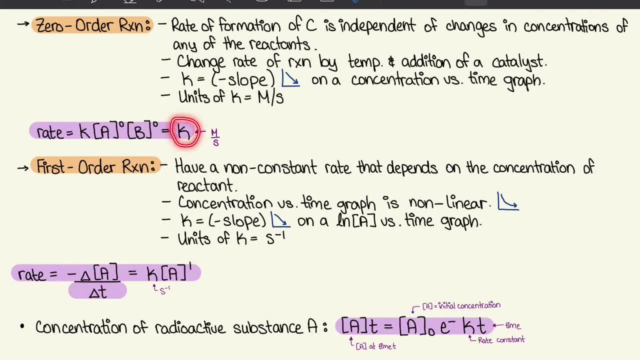 So the rate is just the rate, constant And that's that. So, moving on to the first-order reaction, now they have a non-constant rate that depends on the concentration of the reactants. So the concentration versus time graph is non-linear. 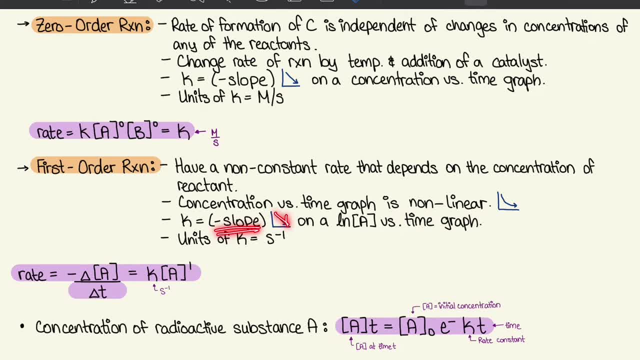 And the k also has a negative slope on a ln of concentration. So the concentration with A versus time graph And the units for a first-order reaction, the units for k, is S to the power of negative 1. So down here below we have the equation for that: where rate is equal to negative, delta A over delta T. 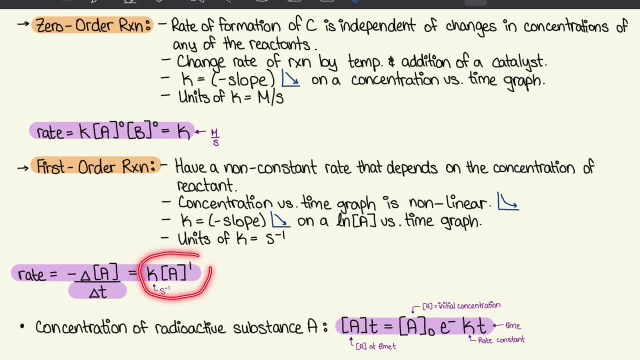 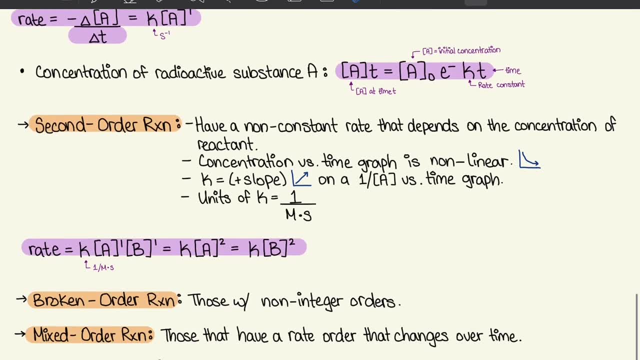 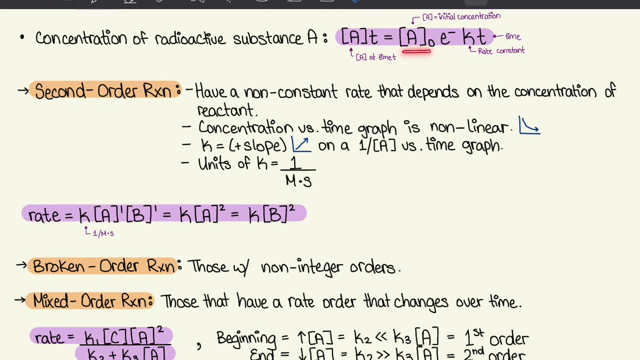 And that's equal to k with the concentration of A to 1.. And the units for k would be S to the power of negative 1.. So the concentration of a radioactive substance- A1. would be AT- is equal to A initial E minus kT. 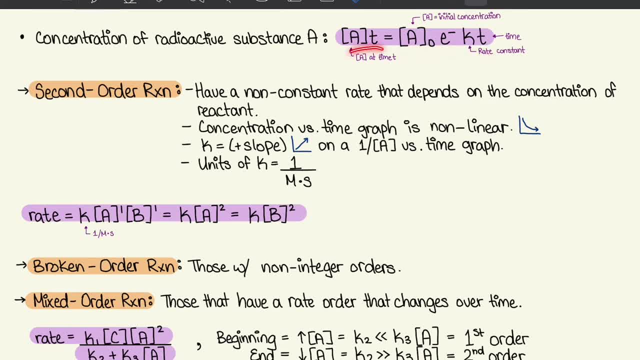 So AT would be the concentration of A at time, E And A0 or A initial would be the initial concentration of A, k would be the rate constant and T would be the time. Moving on to the second-order reaction, they have a non-constant rate that depends on the concentration of the reactant as well. 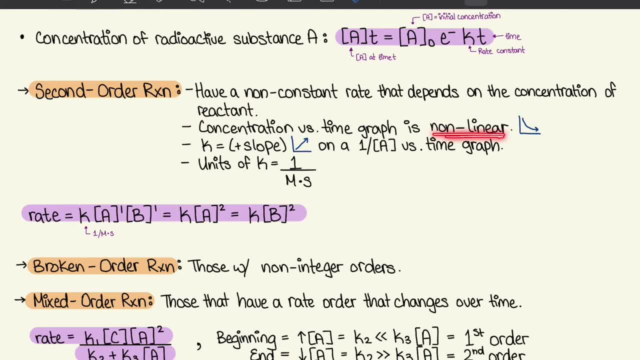 So they have a non-constant rate that depends on the concentration of the reactant as well, And their concentration versus time graph is also non-linear. However, the k has a positive slope on it- 1 over A versus time graph, And the units for k in this second-order reaction would be 1 over molarity times. second. 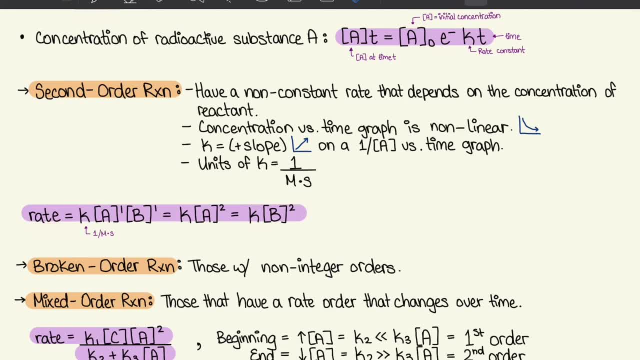 And down below I have the equation for that. You can either have rate is equal to k, with a concentration of A to the 1 and concentration of B to the 1.. Or you can simply have the constant with a concentration of A to the power of 2..